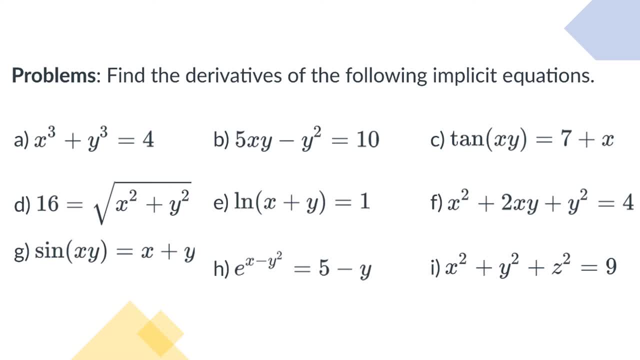 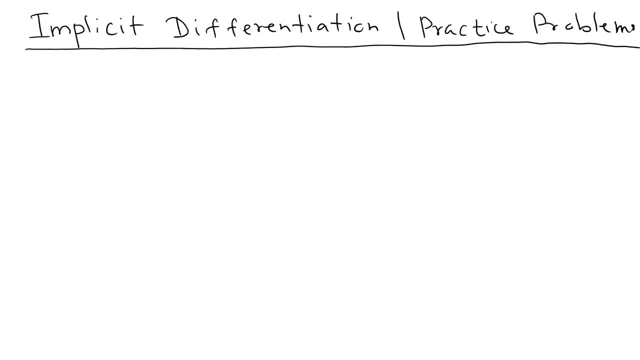 your answers with the solutions discussed in the video. thank you. so take your time and try to find the derivatives first. in this video we do some practice problems for implicit differentiation, so this is a short version of the video. so try to watch this video after watching the main video. 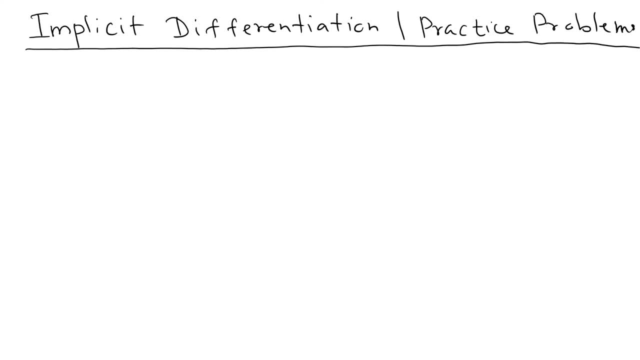 about the implicit differentiation and the long version of the practice problems, which discuss more details. so, uh, when you do implicit differentiation, we have remember two things. first, we gonna differentiate both sides of the equation. so that's one thing, because there are two. this is equation, so we can differentiate. 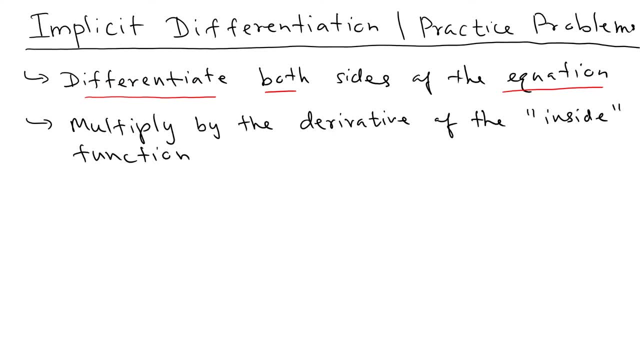 both. next, we then multiply by the uh, by the derivative of the inside function. so you know, uh, what mean by what is mean by the inside function. if you watch the video about the chain rule, that discuss more chain rule type problems. okay, so let's look at the first problem now, actually before that. 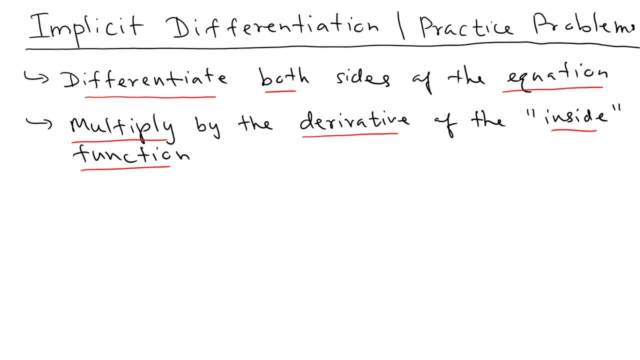 we have some notations that we can use. for the derivative of the inside function. we commonly use dy by dx and also to save time we use the prime notation. so that's like most common in problems, the prime notation, and also it can be like, let's say: you uh, differentiate z variable. 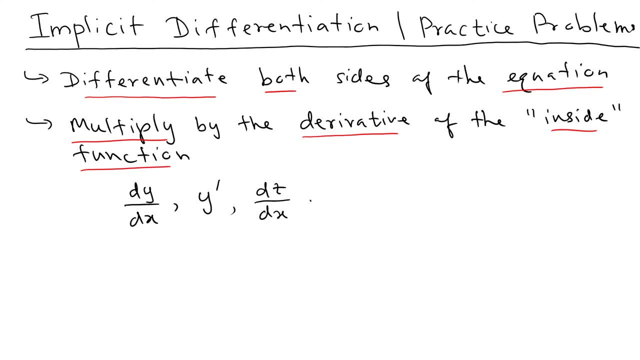 with respect to, so you have dz by dx. also sometimes it's very important practice problems like you take the derivative with respect to time, so it's like d by dt. also we sometimes use the expression, especially when you take the derivative respect to a time, we use the dot notation, so it's like 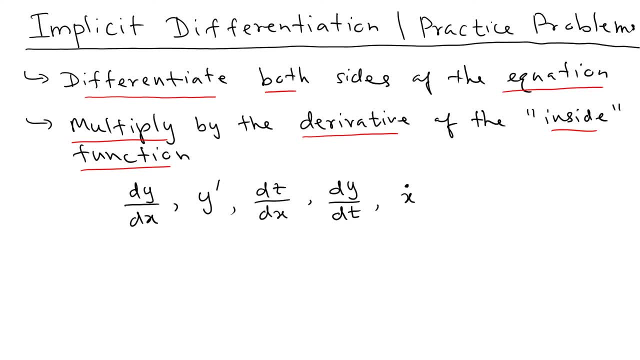 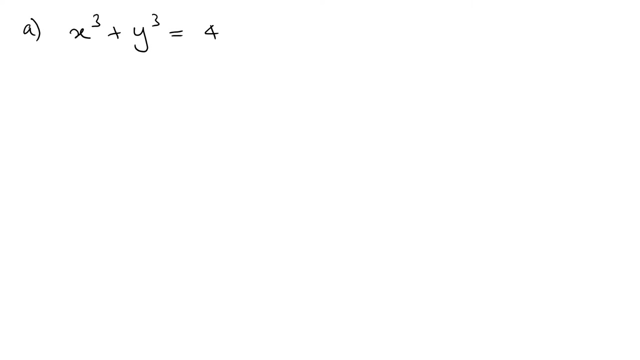 x dot. so so those are the common things, that we use, this one especially for time variable. so when you take the derivative with respect to time, we use a dot to distinguish it from the uh, the prime. okay, so let's look at the first problem now. as the first problem we have x3 plus y3, equal 4. 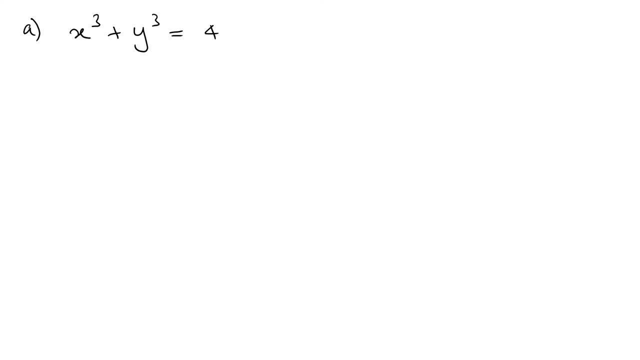 um, so what we do? so you have to say which variable we can use. so we're going to say a differential uh with respect to, let's say x. so you have a lot of options. you can say x, y or even time, like t variable. so let's say x. so if you do that, so we just use the power rule. so we know the. 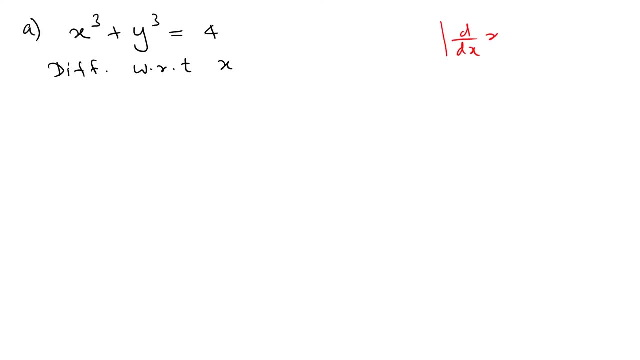 power rule. so that means, uh, if we have x to a constant, this is simply n x, n minus 1.. so we're use that now. so if you use that, we get 3 x squared and then so that's derivative with respect to x plus. you can see, the next term is not x, it's a function of y. so what we do, we 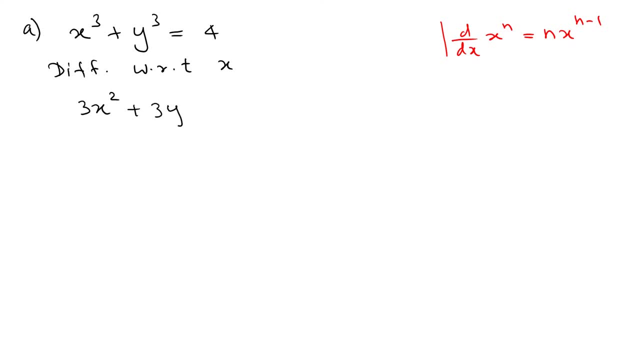 just take the regular derivative, like 3 y squared with respect to y, and then we multiply by the derivative of the inside function. in this case it's a d y over d x. so you can see that this is the application of the chain rule. so, this coming from the chain rule, 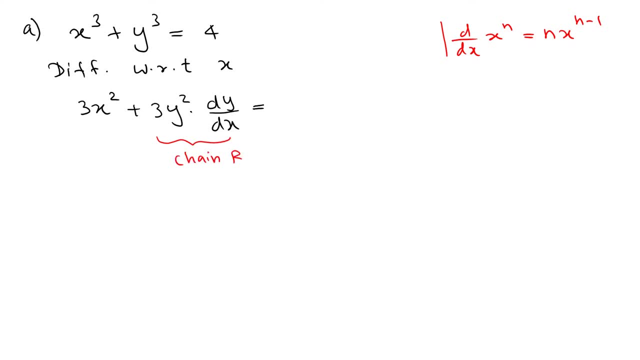 so this is chain rule. so, since you know, uh, since you watch the video about chain rule, you know clearly what's going on here. so, um, and then we have a zero on the other side. so, uh, if you recall the chain rule, uh, what's the chain rule says? if you, 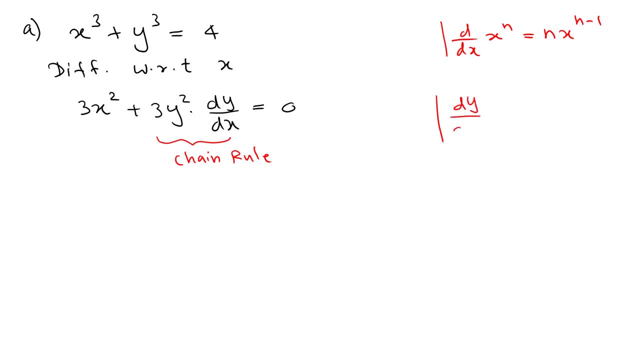 want to take the derivative of y with respect to x, but we um. what we can do is we're going to rewrite this function using a u variable, so it's a d y over do u? we take the derivative with respect to u and then multiply by du over dx, so that's the chain rule. so 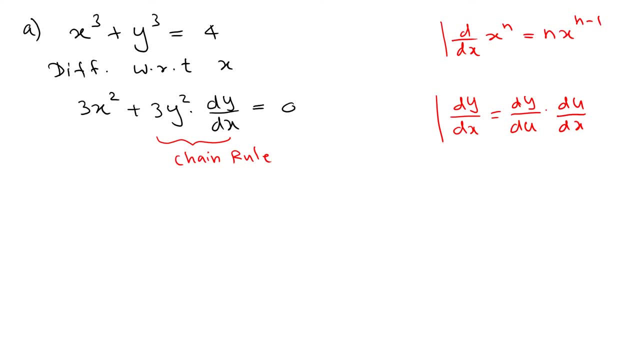 that's exactly what happened here, um, so here the inside function is y. so so this part, uh, actually produce 3 y squared, and now we can cancel 3 because that's common. so we divide by 3 both sides, so you're going to get x squared. 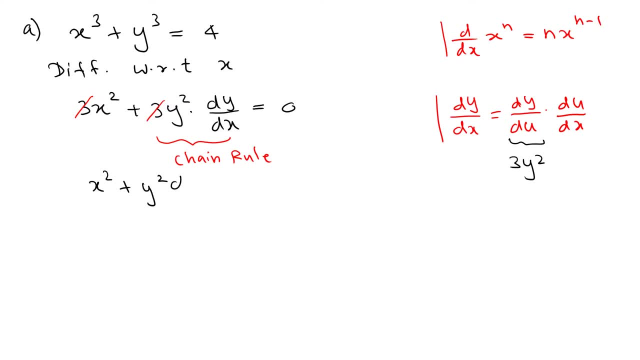 plus y squared equal times d y over dx equal 0.. now we can isolate the derivative term. so what we do? we're going to move the x squared term to the other side. that means we can write this one as x squared. d y over dx. equal negative x squared because 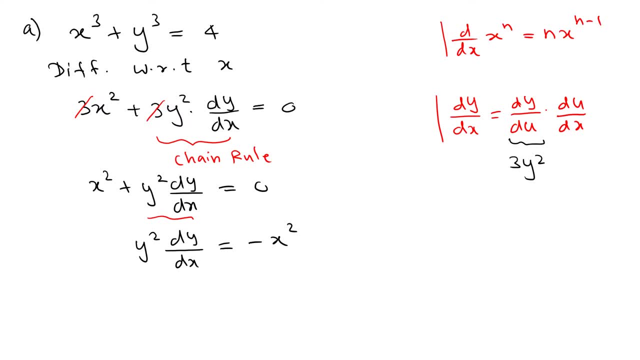 when you move a term to the other side, simply switch this side- so that's the easiest way to remember this- and switch the sign. now we can divide both sides by y squared, so you're going to divide both sides by y squared, so you're going to get d? y over dx, equal negative x squared over. 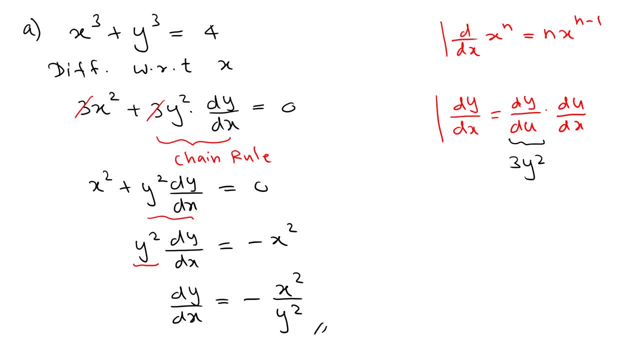 y squared as the derivative. so it's it's not that difficult. so let's look at the next problem. so, as the next one we have, 5 x, y minus y squared equals 10.. so you can see that there's a product here. that means we're going to use the 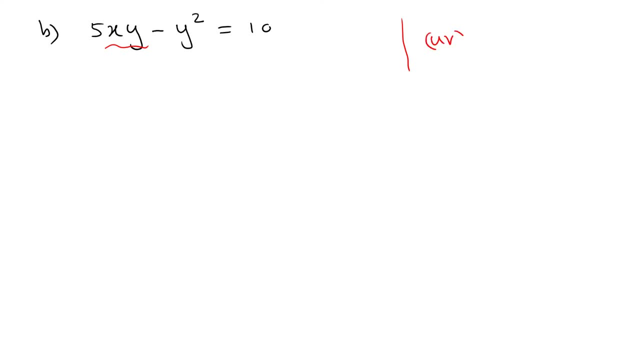 product rule. so, uh, so the most common version of the product rule is: we can write this one as v u prime plus u v prime. we use this version because you can see that if you look at the quotient rule, you can see it's the exact same. 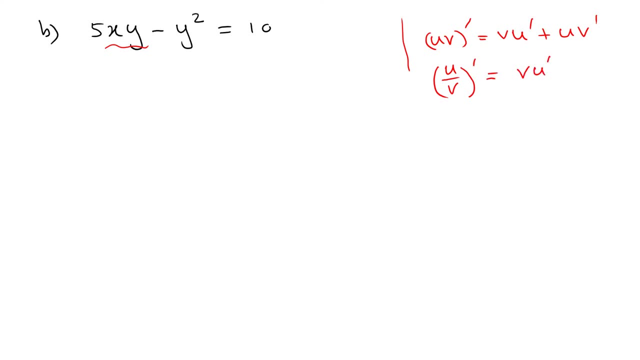 top term. only with the slight change you have a negative sign. so that's why we remember that as a product rule. so this is the quotient rule. this is exact same term, but with the minus sign and then v squared. so if you remember this way, it's much easier to remember these formulas. 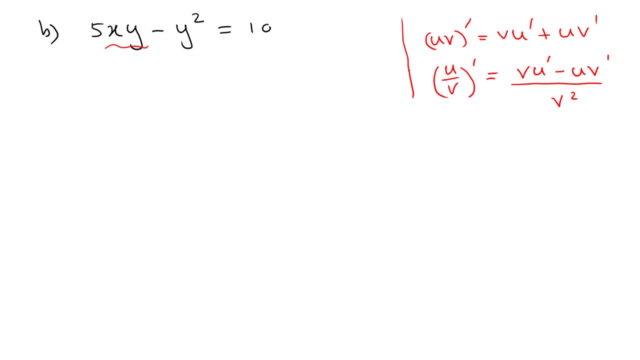 uh. so it's the same term of the numerator with the sign change. that's it, okay. so we're going to use that here now so we can say uh. so we can take the difference uh, different set again as before with respect to x. you have to write it because you have. 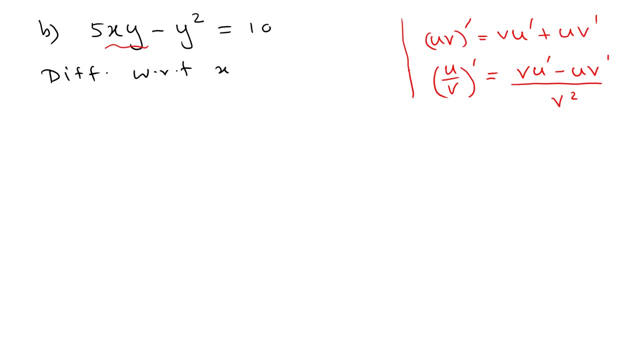 two options here. if you don't write it, it's not clear what you're trying to do, so we write it, always with one derivative. okay, so it's five, which is a common one. we can take it out and then use the uh product rule here. so here's the product rule. what do you get? 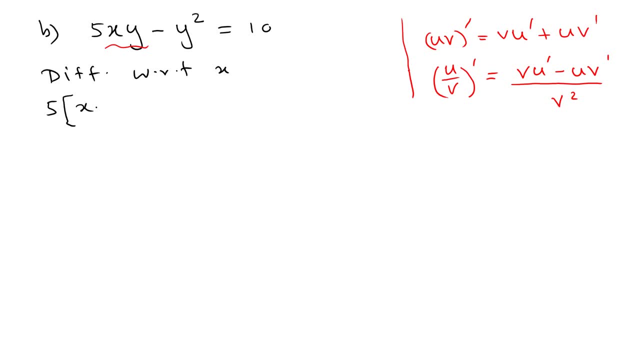 the first term and take the derivative of the second one, so it is d y by d x plus y, and then take the derivative of the other term, which is one. so that's what you get as the derivative of the product. it's always same. that's not going to change. 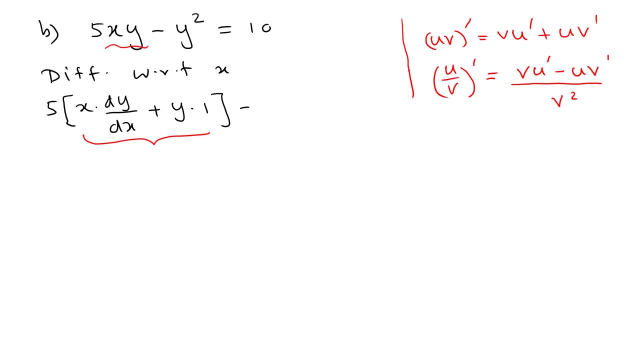 and the minus. we have a function of y, so we take the data with respect to y first and then we multiply by the derivative of y, because it's not going to change. you know, uh, it's a constant, so it's here, okay, so you cannot simplify, there's nothing, uh. 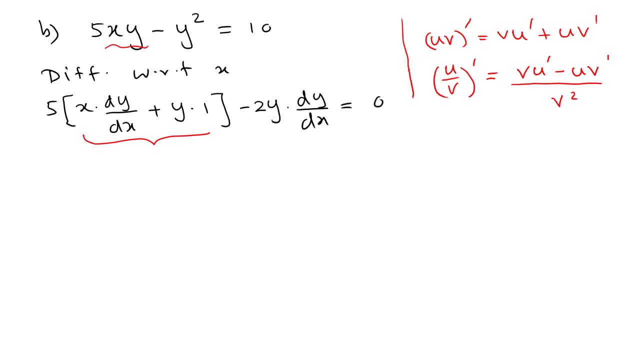 no common terms there. so what we normally do: normally we distribute this first. so when you distribute, you can see that you're going to get 5 x, d y over d x as the first term, plus we have phi y, equal, and you can see: uh, actually i'm going to write the next term, so we have a minus. 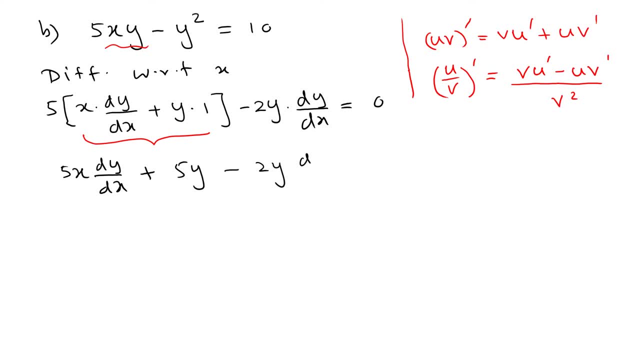 2y, d, y over dx. so what we normally do is the next step. normally, after distributing, normally what we do we're going to collect the derivative terms and then move the terms without uh derivative to the other side. so that means we can write all of them at once. so normally, like in this step, 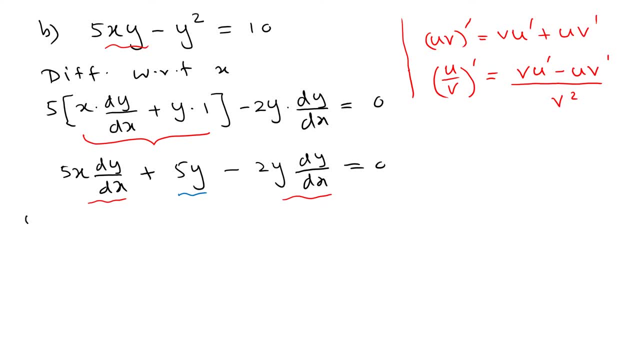 what will happen is the cancel�� raze. so cancel common factors, cancel common factors. that's like a theoretical step. so we do that here. just to uh simplify this: cancel this is there are no common factors in this case. we're going to skip that step. so what we're going to do 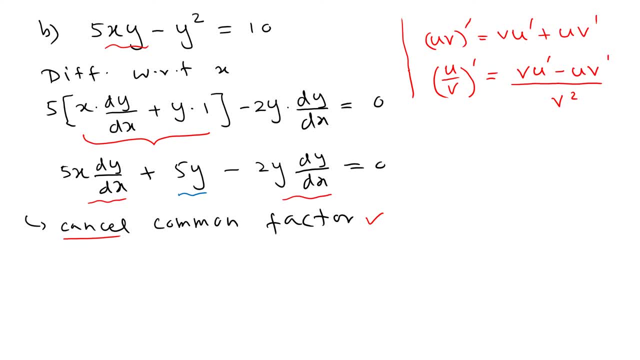 is: uh, we're going to take the terms with derivative, so we're going to collect this, so we have 5x d y over d x, and then we're going to move the other derivative term here and then we can move the terms without derivatives with other side. so we can write it like that. now what? 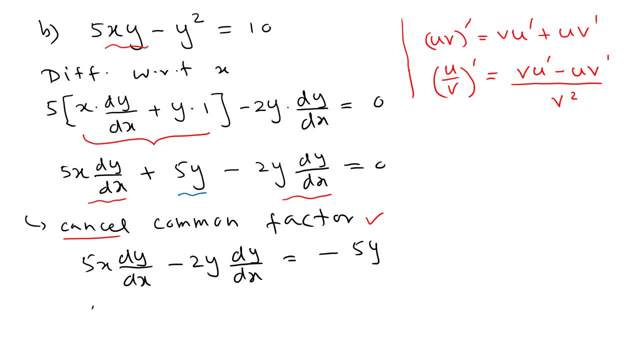 we're going to do? we're going to factor out the derivative. so that means you're going to get 5x minus 2y. we factor the derivative, it is d y over d x, so we have negative 5x, uh 5y, so we have negative 5x 5y. 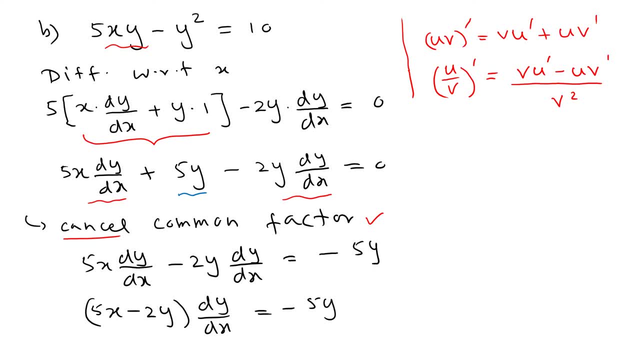 so we have negative 5x 5y, so we have negative 5x 5y, negative 5y, and then what will happen is you can divide both sides by that factor, so that means you're going to get d y over d x, equal negative. 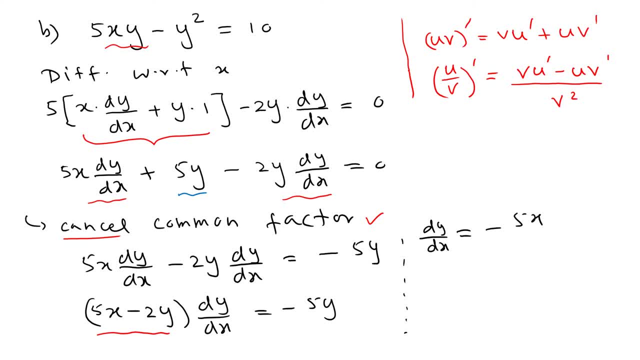 5x 5y over, 5x minus 2y. um, i mean there's nothing, but you can see there are two negative signs. but if you multiply the top and bottom by negative, you can write this with a less number of negative signs. so i'm going to multiply top and bottom by 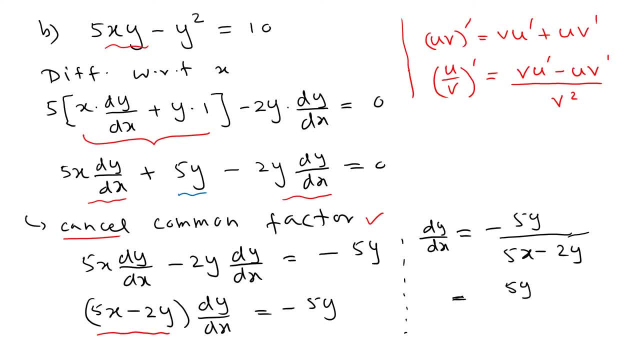 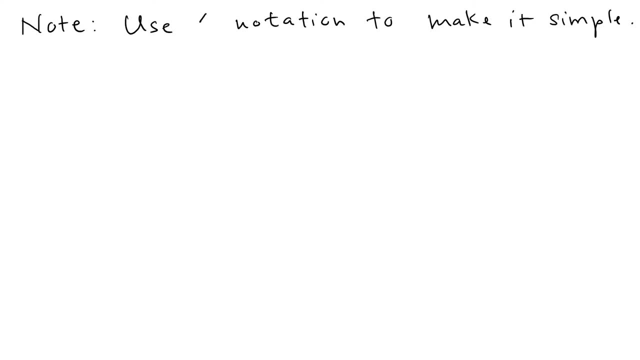 negative, so you're going to get 5 y over 2 y minus 5 x, so that is much better than the previous one, so we will write it like that. okay, let's look at the next one before we start the next problem. before we start the next problem, actually we have a not, so what we normally do is we can use the. 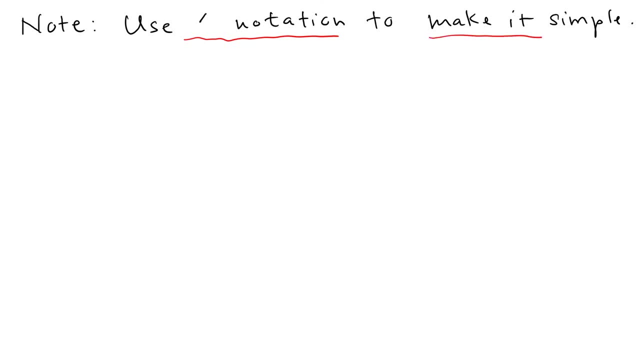 prime notation. because the prime notation? to make it simple, because you can, when you supply notation, you can reduce the unnecessary writing. so let's look at the next problem with the prime notation now. so we have uh, tan x, y equal x plus uh 7 plus x. so here we have one more thing we also need to. 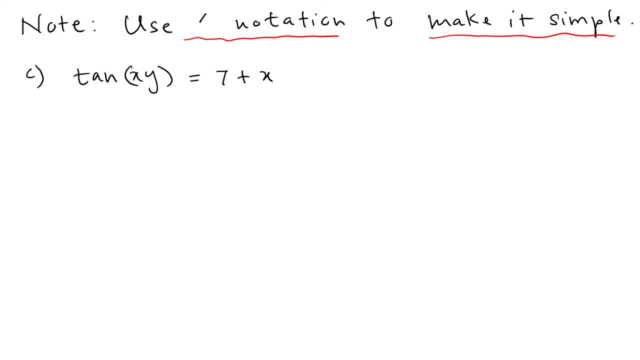 know, like, when to use the parentheses and when not to use the parentheses and wait. next it is not necessary. so in this situation you have to use a parenthesis, because if you do not write the parentheses, this may be a different problem. so the problem may be: tan x times y. so we deserve. 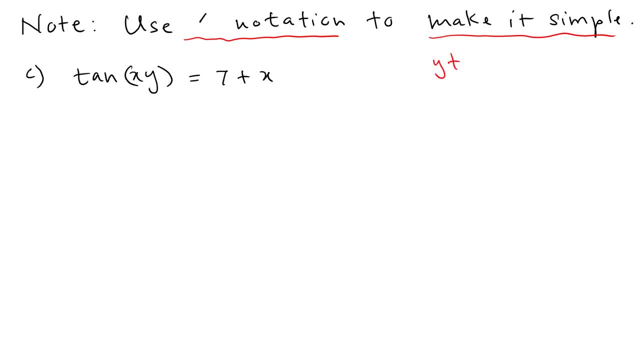 that's a different problem. that's like y times tan x, so that means this is not equal to tan x, y. so you have to be very careful what we really mean by this. so if you mean x as a single product, it will be better to use the parentheses. so 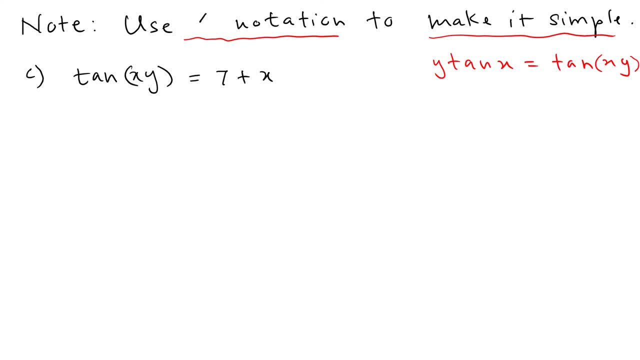 so very be careful, like how to use and when to use the parentheses properly. so you can see this is here. we need the derivative of tangent. so let's recall that. and we know that the derivative of tangent, derivative of tangent, is secant, squared x. so because of that, so if you take the derivative, 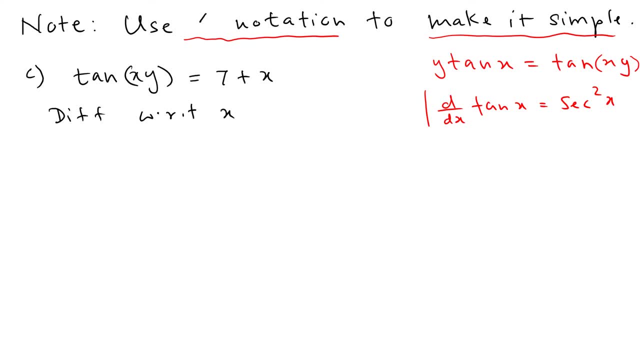 with respect to x. so you can see it is the secant squared. and then x, y- we don't take the derivative, we don't do anything with that- and then multiply by the derivative of the inside function which we already took in the previous problem, which is x, and then 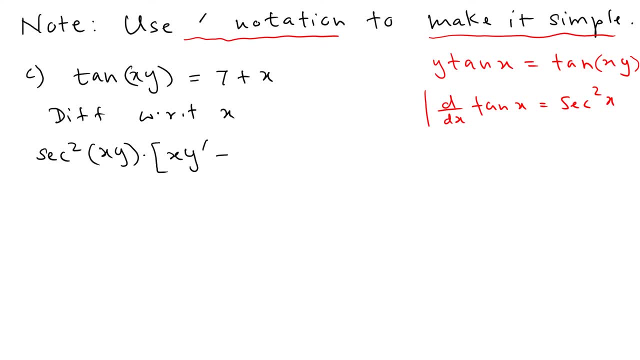 take the derivative of the second one, which is y, prime plus y. take the first one, which is 1, so that's what you get. so this is the derivative of the x? y product. that's the derivative of the x? y product. okay, and then equal the other sides. uh, 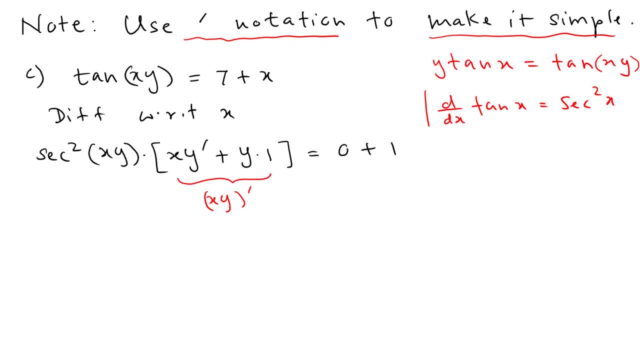 7 is a constant plus 1. okay, so as uh. so the next step is: we see whether there are any common factors. there's no common factors, so what we do next is we're going to distribute, so we distribute. you're going to get secant squared x y times x y, so it would be better to write x- y in front. 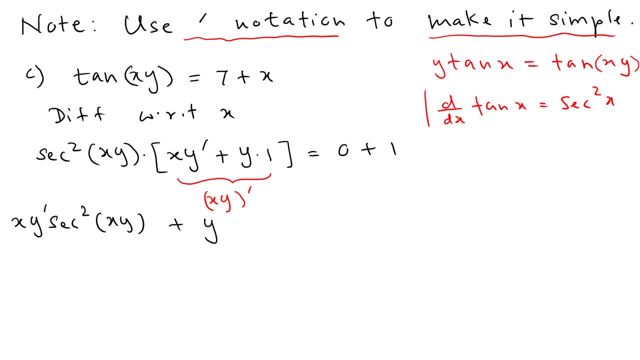 just to avoid confusion. and then y. we write that in front, secant squared: x y equal 1. so what we do next is we're going to move the terms without derivative terms- that means this term- to the other side and then divide by the factor. so. so that means next step would be x y prime. 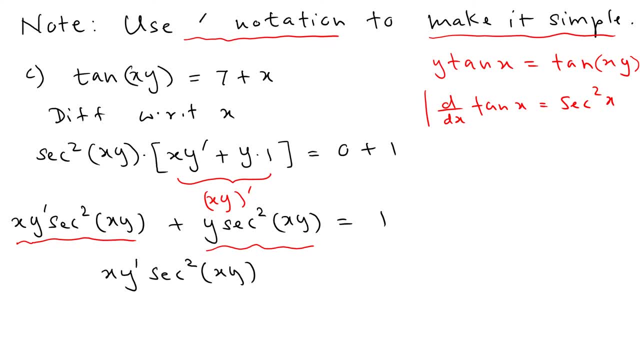 secant squared x y, which is equal to 1 minus the other term. and then we're going to divide. we're going to say y prime equal 1 minus y secant squared x, y over, we have x secant squared x 1. so that is the derivative. 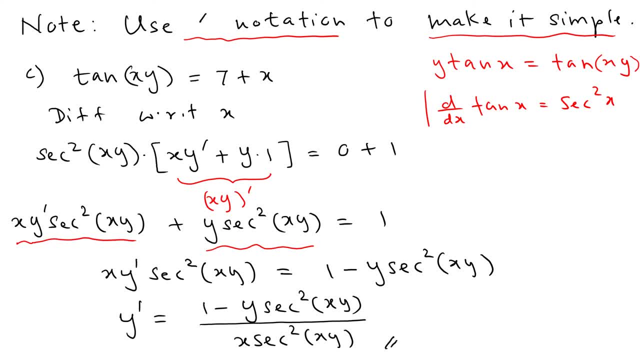 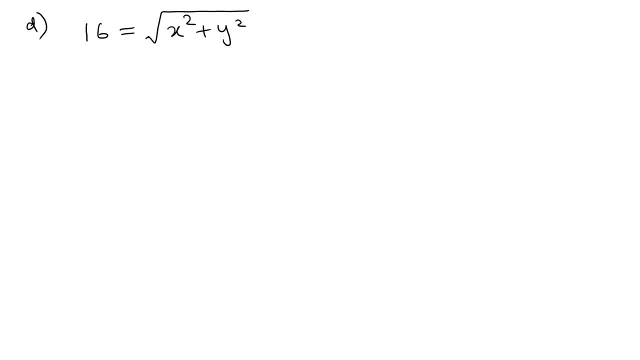 you get. so let's look at the next problem now. next, we have 16 equal x squared, plus y squared equals square root. you can see this is another way to write the equation of the uh circle. so what? so you can see that this is simply uh. 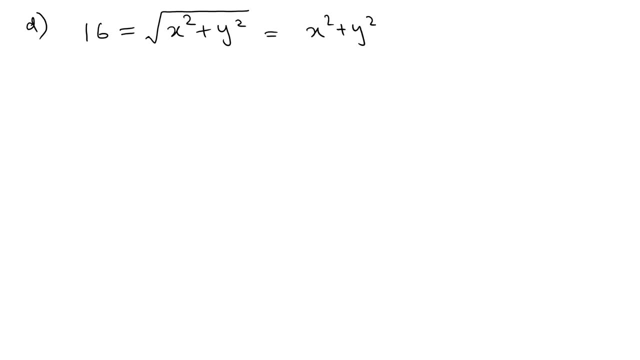 you can write this one as: x squared plus y squared to the one half power, derivative means the one half power. square root means one half power. what we would do normally is we're gonna uh, square the equation. both sides so square, in both sides, so squaring. 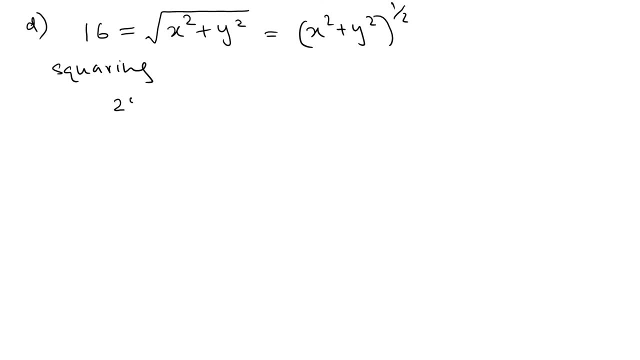 we're going to get square of 16, which is 256 equal if you square the square root, and we know that it's going to get cancelled out. it's going to cancel out. so this is what we get, because you can see, this is much simple to work with. in the long video, actually, we discuss what 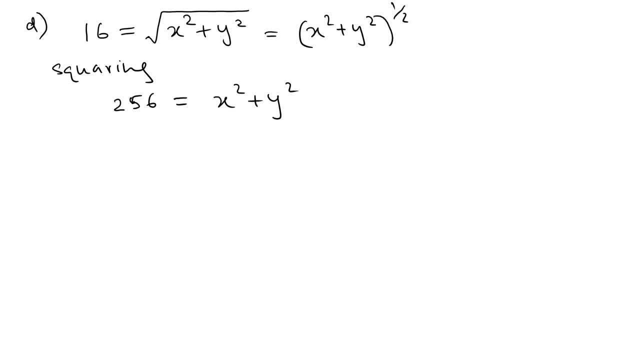 if, if you do not do that and you can see that the expression get a little complicated, but at the end you get the same answer, so please look at the long video about another way to like get the answer without doing it. uh, so now what we can do: we're gonna take the derivative with respect to. 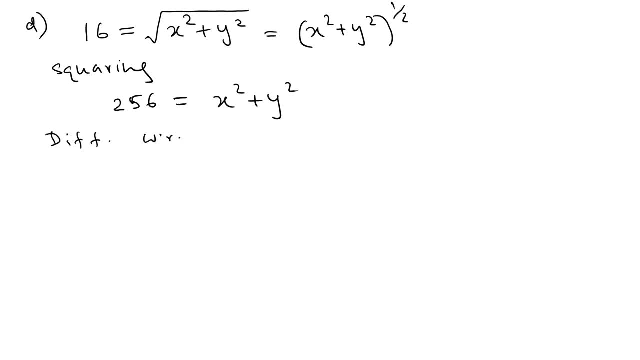 x. so we're gonna differentiate with respect to x. so you're gonna get zero on this side as a constant. the other side, x squared, which is 2x, and then this is y square. so we take the derivative to y first and then multiply by y prime. 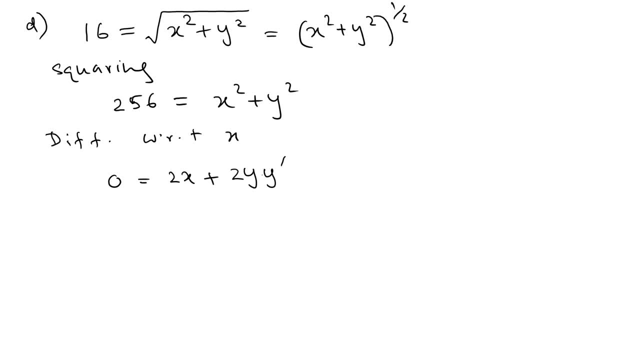 so that's what you get. now. what we want to do is we're going to solve for y prime. this is very easy to solve for y prime. so y prime is: first we're going to move the 2x term, the other side, which is negative 2x, and then divide by 2y, so in which you can simplify, cancel into x over y. so 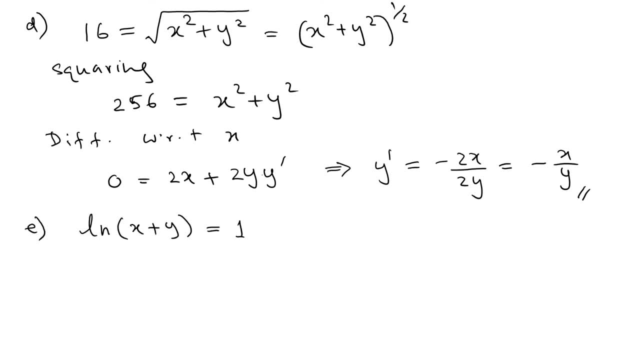 that is the derivative of this one, uh. next we have ln, x plus y, equal one. so, uh, we need derivative log. so we know that derivative of a natural log is one of x. uh, even with the absolute sign is the same thing. even if you put the absolute sign is the same thing. so, uh, if you use that uh again, uh, differentiating. 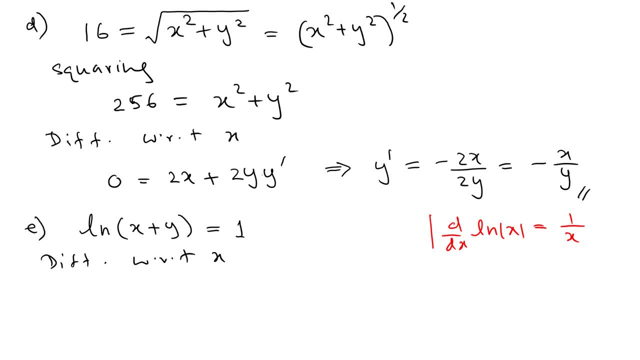 uh, with respect to x, just make it a practice, so just to write like better math. so, uh, so the inside function is x plus y. so according to the formula, one of x by x plus y goes down, and then the derivative of x plus y, which is derivative of x, is: 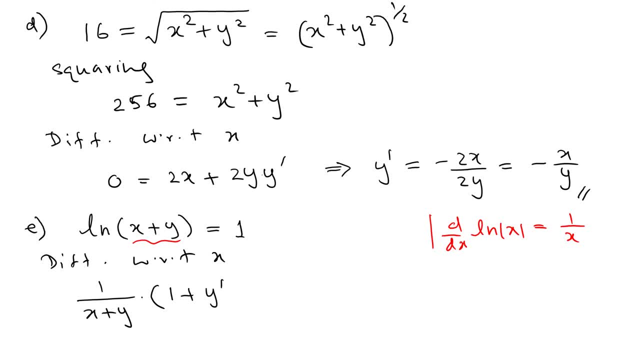 1 derivative y is y prime equals 0, and then what's going to happen is there's a 0 on the other side. that means we can: if you multiply both sides by 1, over both sides, by x plus y, this is going to be 1 by 2x. 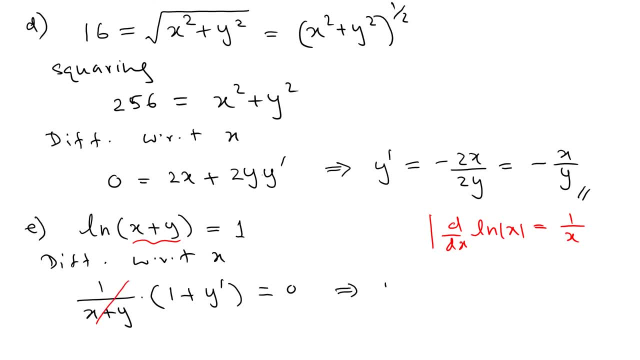 that means you simply get 1 plus y prime equals 0. this is that y prime equal negative one. so that's very interesting. so let's look at the next one. as the next one, we have x squared plus 2, x, y plus y squared equal 4. again, this is a implicit function, with respect in implicit function of y. so we're. 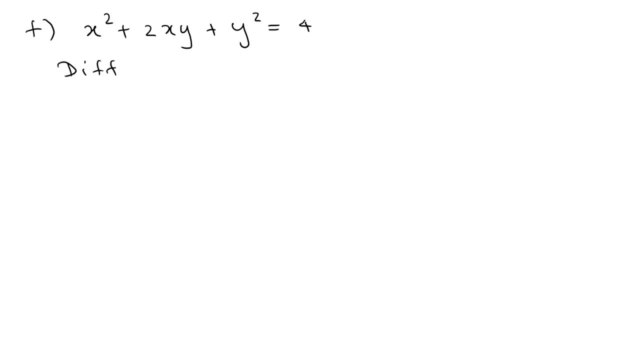 going to take the derivative uh with respect to x- uh. so if you do that you're going to get 2x and then we have the product. so when you do the product, you can consider this as one function and then y is another function. so that means i go to. 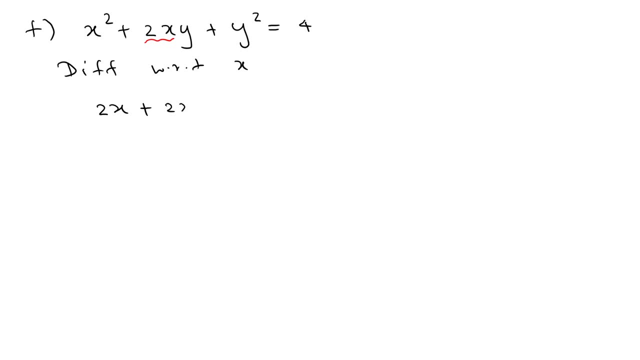 the product rule. it is the first function multiplied by the derivative of the second function, and the second function is the derivative of the second function multiplied by the derivative of the first function, the certificate. so that's the derivative of the x- y product and then plus y term. so we take the derivative with respect to y and then y prime. 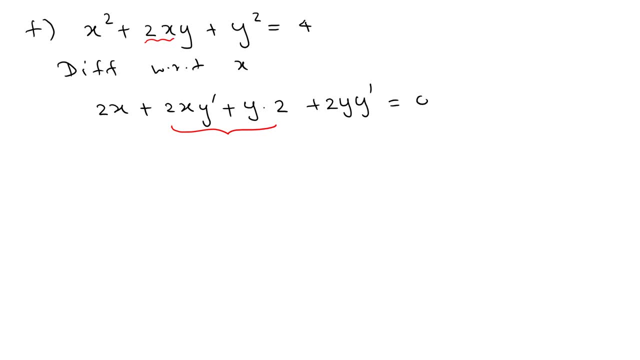 equals zero. uh, what we do next is we can cancel the common factor, which is two, so we can remove that, and then we're going to combine terms with derivative on one side, terms without derivative on the other side. so if you can do that, you can get the derivative of the first function. 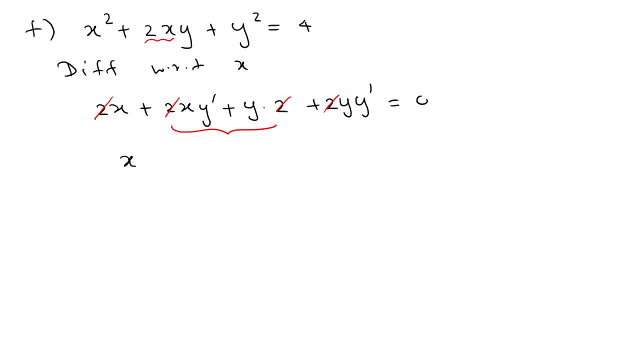 y prime terms, you can see that you're going to get x plus y, y prime equal. if you move the terms without x to the other side, you're going to get negative x and negative y. if you factor negative sign is x plus y. oh, this is interesting. uh, you can see that. 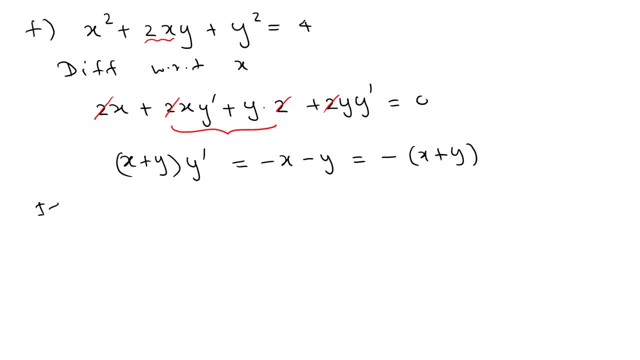 if if x plus y not equal to 0, you can just cancel that term not equal to 0, then you can cancel this term, because if x plus y equals 0, you cannot cancel, because 0, 0 equals 0, um. so that means this this: 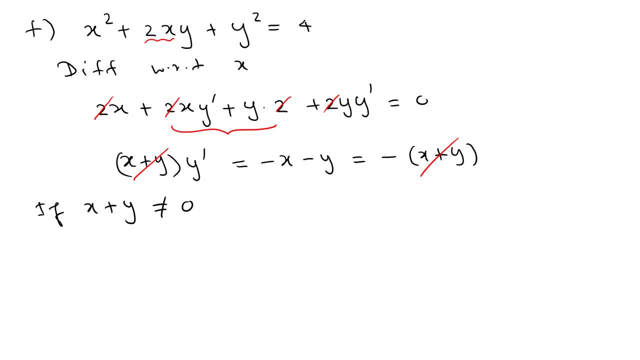 what we're trying to do is not valid for any point on that line, which is the line uh. you can see, this is the line x, y equal negative x, that line. so if you have anything on this line, so this formula is not valid. that's why it says: 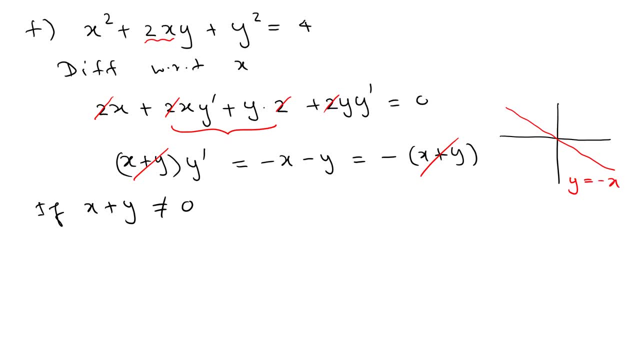 you? okay, so since if this is not the case, we can write this one as y prime equal. uh, you can see that it is negative 1. it's kind of strange and you get the same answer again: negative 1. so, but you can see, in this expression there's no x, y terms. 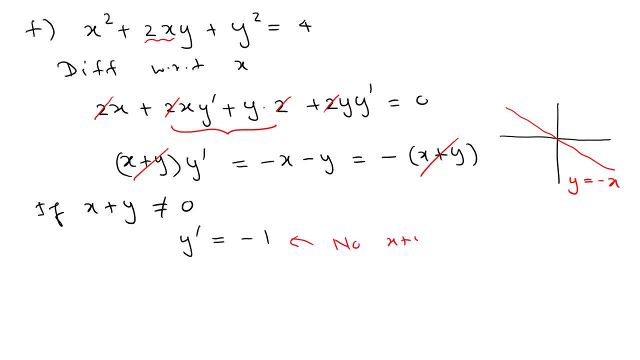 so no x plus y, uh term here, uh. so that means there's no issue here. so that means the derivative of uh, this uh, the with respect to the implicit derivative is negative one. and this kind of strange why exactly happened? and you can see another. look at this one, you can see if you. 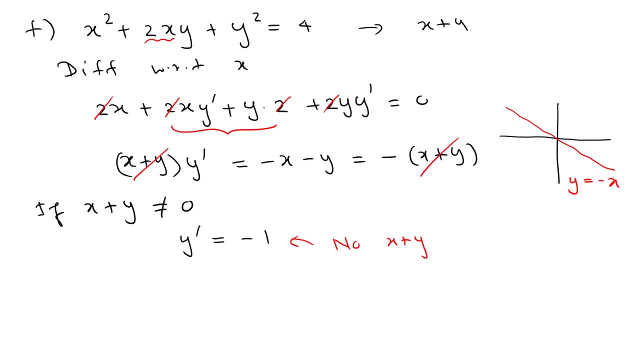 you have a factor, this: this actually means x plus y. whole thing is square equal to four. so if you take the derivative of uh, if you, if you take the square root of both sides, you get um. you can see x plus y, equal plus or minus 2. there are 2 x's and you connect it to plus and it's negative 1. so that goes into negative 1閼. x plus y equals plus, so minus 2. there are two x's and you take the square root of both sides you get, uh, you can see, take x plus y: equal plus or minus 2. there are two x's and you can see this as well. 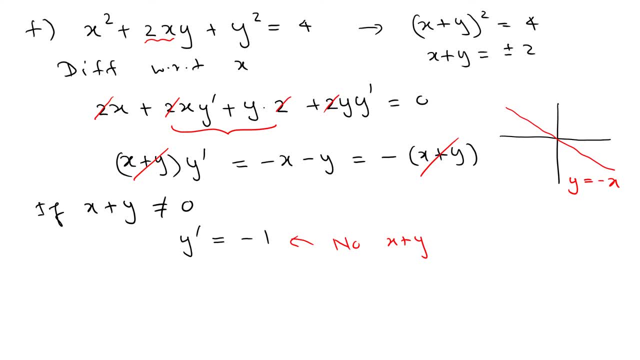 black and white under control 177: 00 and if you have some factors that D x change the language. literally you get a max D x of y equals 1 over 1.. there are two answers. now, if you take the derivative, what will happen? 1 plus d y over d x- equal because the 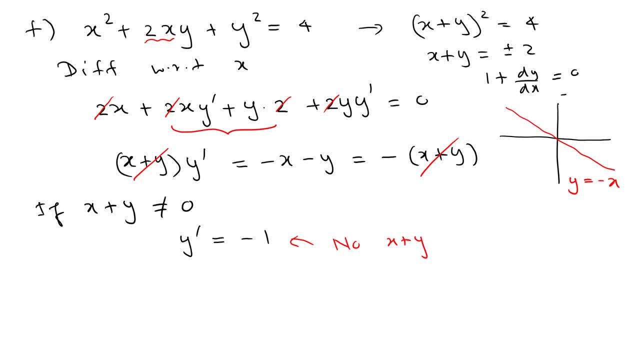 constants are 0, no matter what. so this says that d y over d x equal a negative 1.. so that's exactly what happened. so what we did is we put two equations, uh, in one formula. that's exactly what happened here. so what we did? there are two equations. 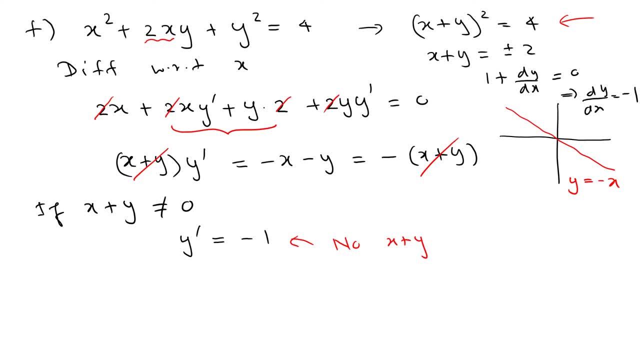 but you write two equations as one formula. it's kind of interesting. so those two equations are: there's one that passes through uh- you can see uh here- at two, the other one that passes through negative two. so what we do? we find the the slope of both line at the same time. 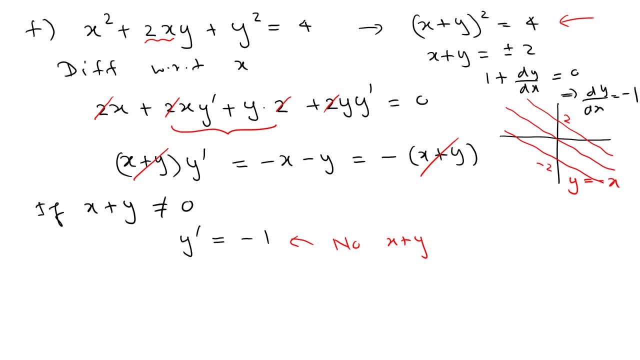 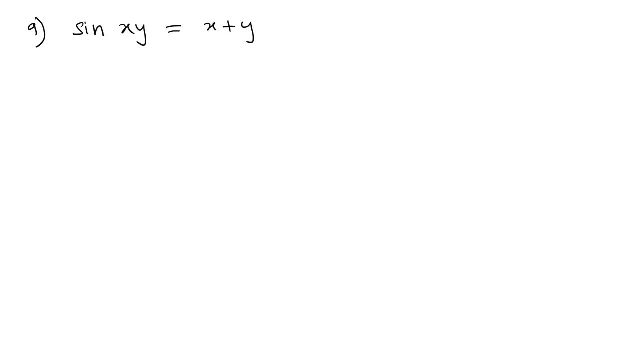 so you can see they all have the same slope at negative one. okay, so let's look at the our next problem. so that's the next problem one. we have sine x, y equal x plus y. just to avoid confusion, let's say we need the whole product here, because otherwise it can mean something. 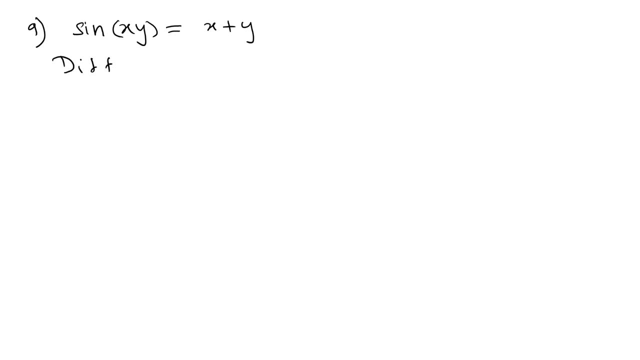 else. okay, now again, as before, differentiate with respect to x. so this is a sine and we know what's the derivative of sine. so derivative of sine is cosine. derivative of cosine is not sine, it's negative sine. it will be very clear if you look at the graph of the functions. okay, 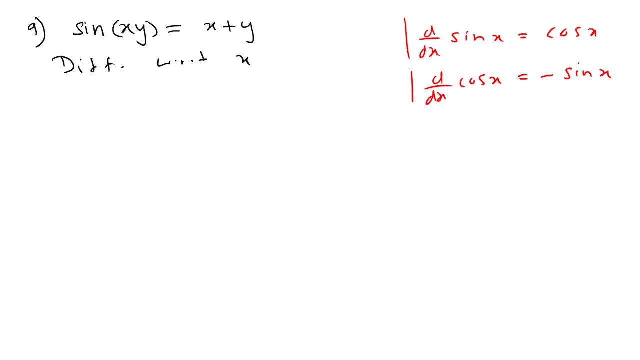 so if you take the derivative with respect to x, uh, now what you get is it's become cosine, the product, and then multiply by the derivative of the product. this we did multiple times. it is x- y prime plus y x prime, which is 1 equals 2. on the other side, 1 plus y prime. now what we do next is see whether 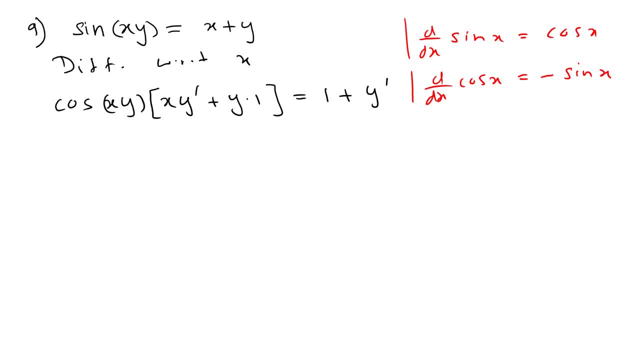 there are any common factors to cancel? no, so what we do is we distribute, so we do is we distribute. and then we also write the those x, y terms in front, so we can write this one as x, y, prime cosine x, y, and then y cosine x, y equal 1 plus y prime. now we can bring the prime terms to one side. 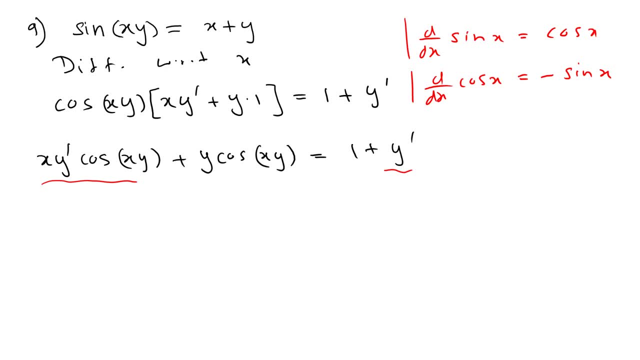 so if you bring the prime terms to one side and factor y prime out, you can see that this is y prime x, cosine x, y and then minus one because y prime when you bring this in minus y prime, so you're going to get that, and then also we can move all the other terms other side, so so it's a sine. 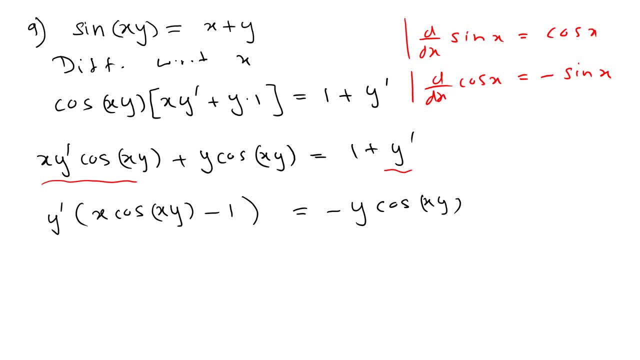 so this is what you get, and then we divide by the factor, so it's y prime equal. you can see, actually there's a one here. so it is one minus y cosine x y divided by x cosine x y. uh, minus one. so that's the answer, and you can see that you cannot reduce. 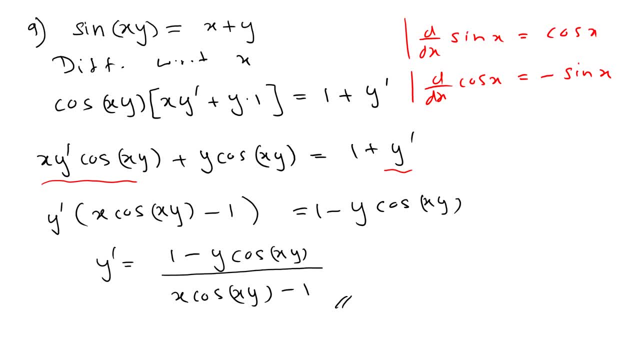 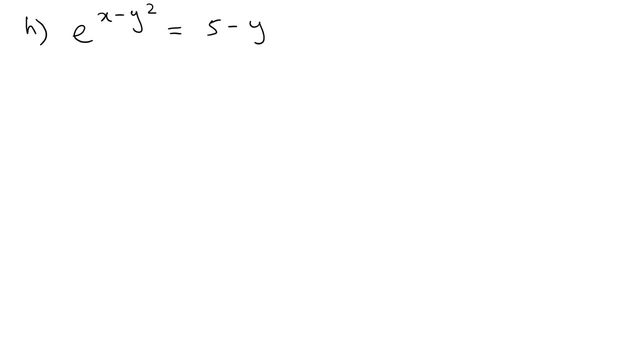 the number of negative signs, even if you switch the sign. so we can leave it like that. so let's look at the next one. as next one, we have a to the x minus y, squared equals 5 minus y. so we use the exponential function and we know the derivative exponential function and we can see that. 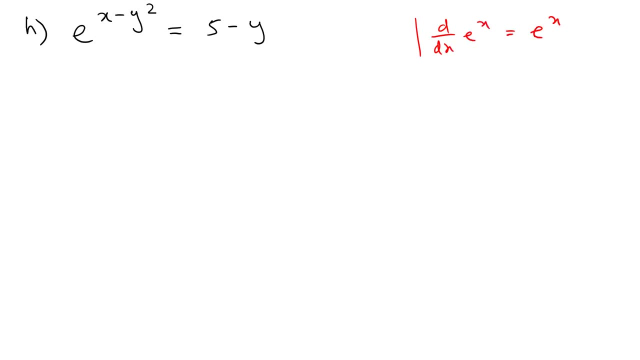 you get e, x back. so uh, so again, uh, differentiating uh with respect to x. so when you have derivative e, so we know that we repeat the function and then multiply by the derivative of the inside function, which is 1 minus 2, y, y, prime. 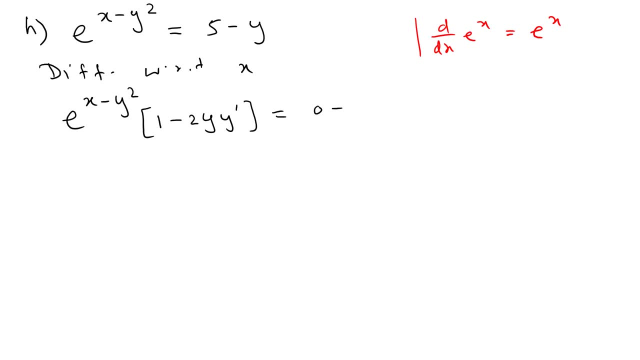 equal to the side 0 minus y prime and then distribute so e x minus y squared minus, we write 2 y y prime in front and then we have negative y prime. bring the y prime terms to one side and factor out y prime. so you're going to see that 1. 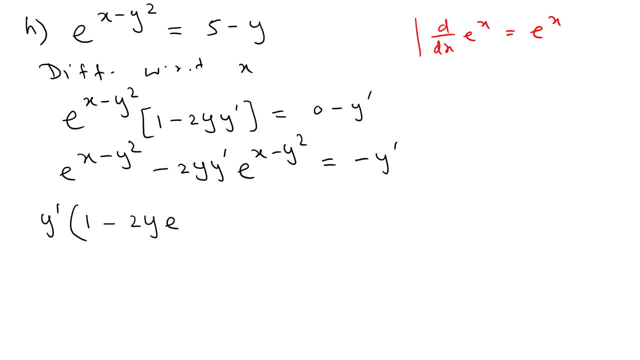 minus 2 y e to the x minus y prime minus y squared. and if you move the exponential term, the other side is going to be negative e to the x minus y squared. so y prime is: if you divide is negative e, x minus y squared divided by 1 minus 2 y e to the x minus y squared. 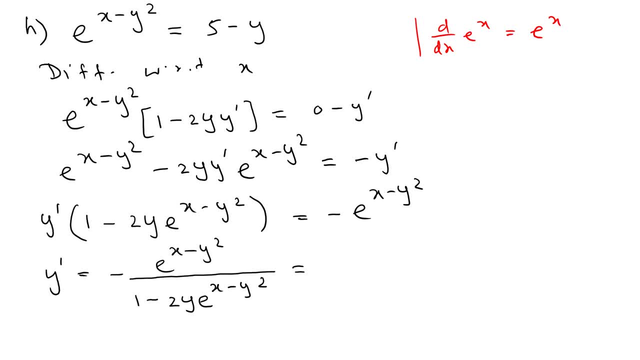 okay, and then you can see that there are two negative signs for this one. so if you multiply the top and bottom by negative, egently you can rewrite this one as e, x minus y squared over 2, y e to the x minus y, squared minus 1. so this is much better than the previous one. 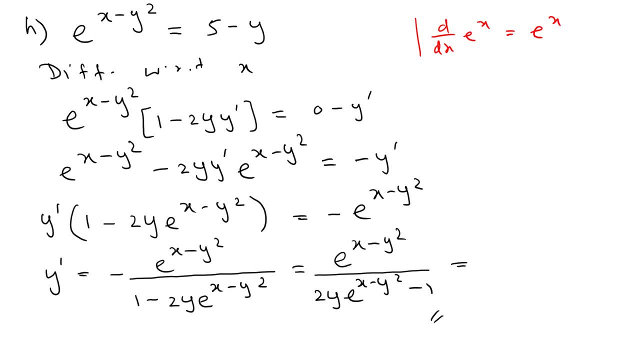 and also, if you multiply the uh top and bottom by e y squared, you can write this one as e x over 2 y, e x minus e y squared. um, so you want to write this one, this one x minus e times options. two, this one times ups: minus x, minus somewhat. so prime over this ci is negative over 2 y e. that's going to be negative ЖÄ, We just. 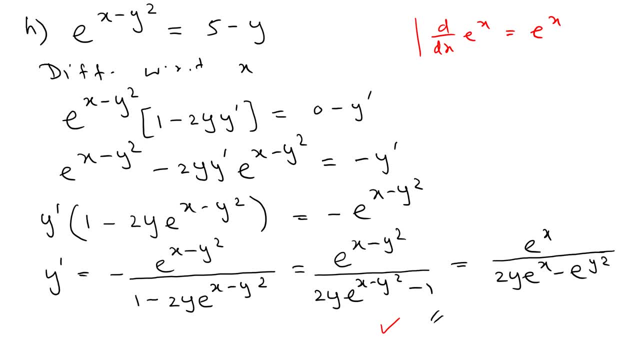 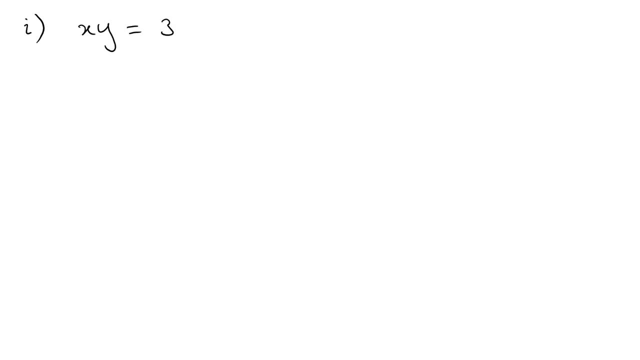 i think, like this one would be much better compared to them, but there are a lot of versions of that. okay, let's look at the next one. so we have x, y equals 3.. so, uh, these kind of equations, uh problem equations, are common. so these are what we normally call the rectangular. 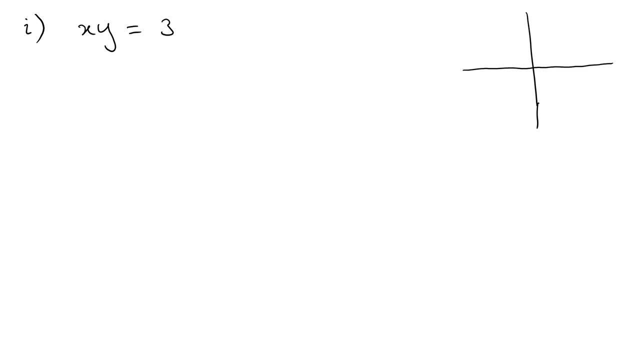 hyperbolas. so that means this is the equation of a curve like this, like that and like this. you can see when one increases, the other, one decreases, um, and also the product is a constant which is equal to 3.. so what we try to do here is like we try. 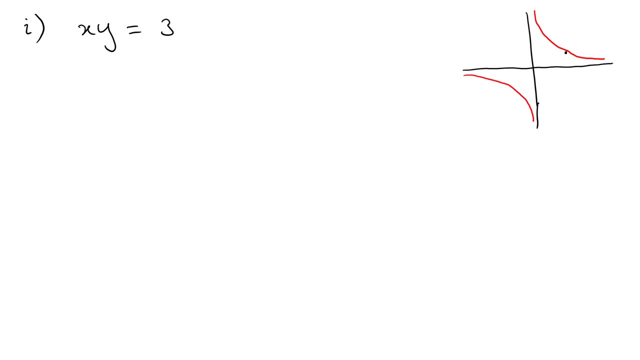 to find a slope, uh, at a point like that. so what is the slope at that point? i didn't go through. well, so like that, so you can find the slope at a point like that, okay, good. so, uh, how we do this? we can just use the um. 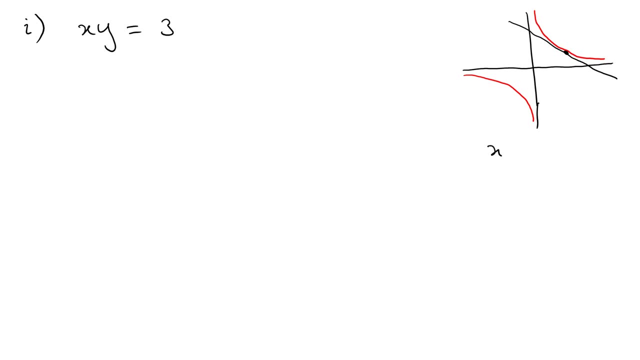 so we can do this problem two different ways. you can write this one as x, y equal 3, so that means y equal 3 over x. now, this is a explicit equation, so you can just take the derivative of this one using the um, either quotient rule or just the power rule. 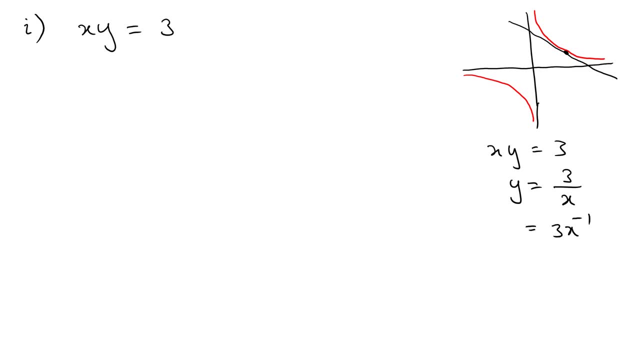 if you use power rule, you can write this one as 3, x is negative 1 and use the power rule. but here we try to use the implicit differentiation. see how you do that. so again, if you differentiate with respect to uh, with respect to x, this is the product and we know the product rule. so it is x, y, prime plus. 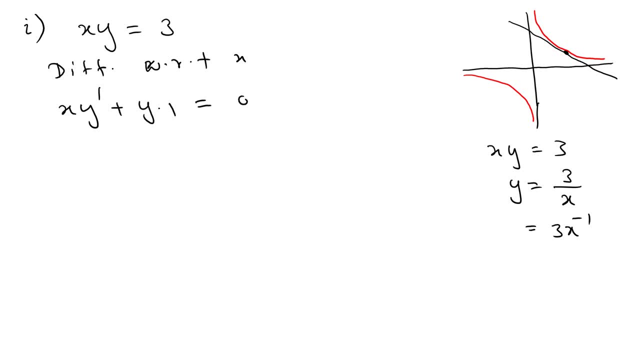 y. x prime equal constant is 0.. so that means y prime equal. you move the y terms to the other side and divide by x. so it's going to be minus y of x. okay, so let's do uh. one last problem. um, how about this? so we have x squared plus y squared equals x. 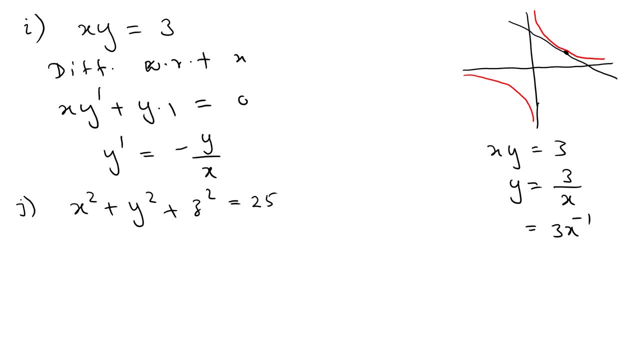 x squared plus y squared plus z squared, equal 25.. what is this? and you can see that this is actually represent a sphere in, uh, three dimension, three dimensional space. so that's a sphere in x, y, c coordinate system: x, y and z. so what we're trying to do is: